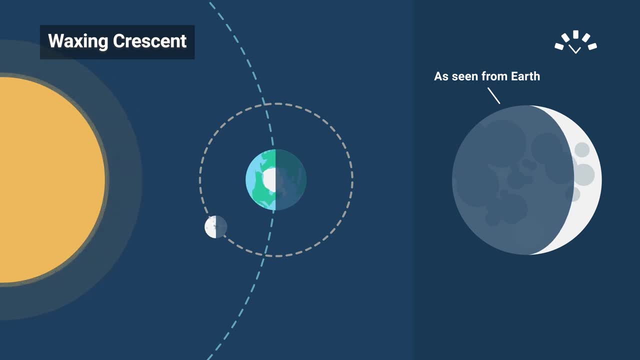 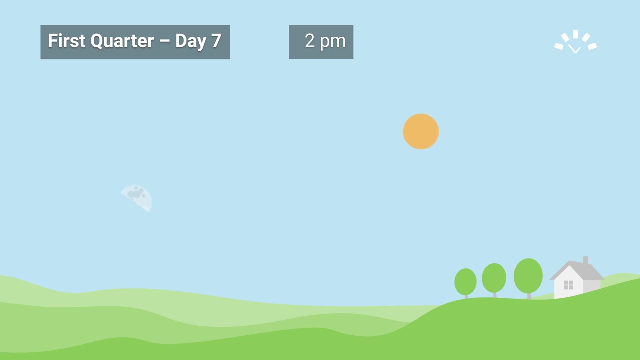 Overall, half of the moon is always in the sunlight and half in the darkness. As the moon orbits Earth, it changes just how much of the lit-up side we can see. A few days later it rises around midday and is visible in the blue afternoon sky. 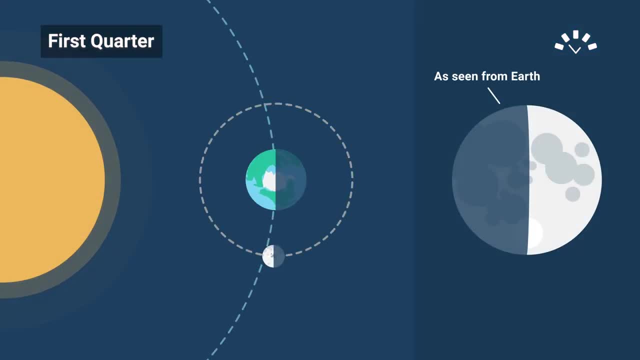 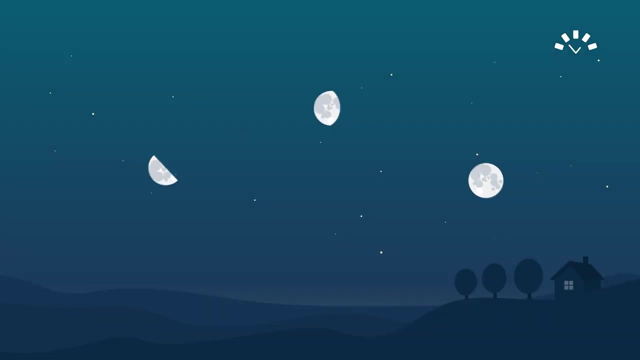 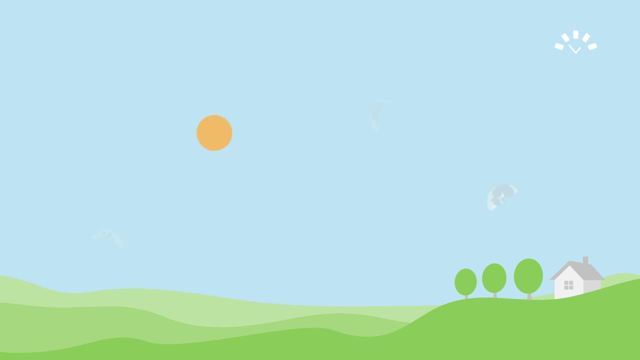 Two weeks later, here it comes: earth. the moon is 90 degrees from the sun and exactly half its face is illuminated. this is the first quarter moon, because the moon has gone one quarter of the way around earth. so what's next? stay with us and see what happens to the moon as it travels through its phases. 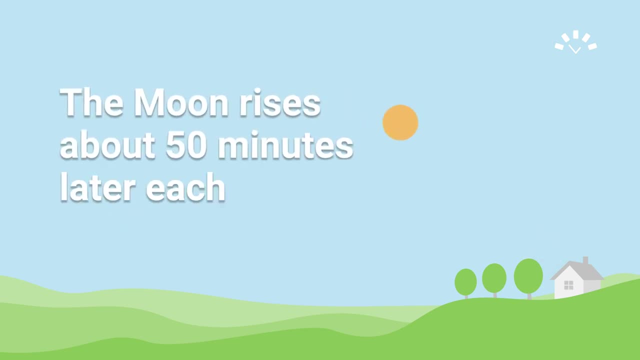 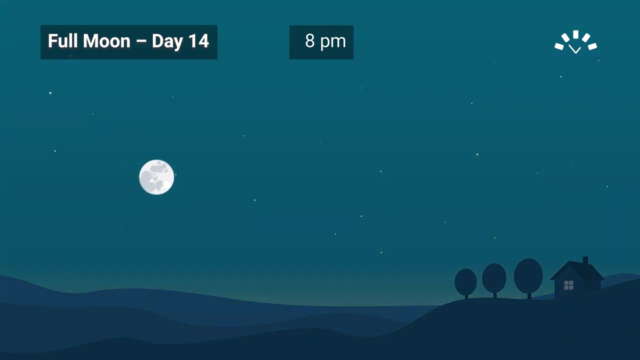 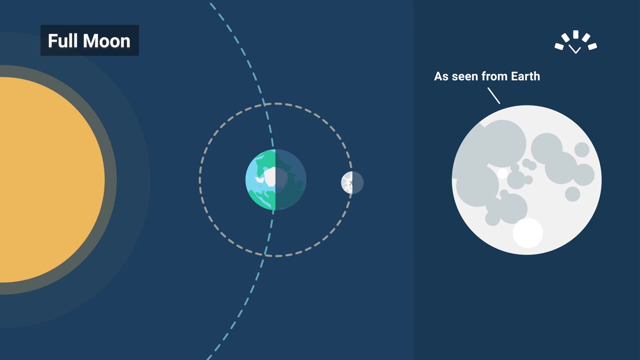 and remember. the moon rises about 50 minutes later each day, about two weeks after new moon is rising at sunset. full moon is the only phase where the moon is up for the whole night. the moon is now on the opposite side of the earth to the sun, and the side facing us is completely 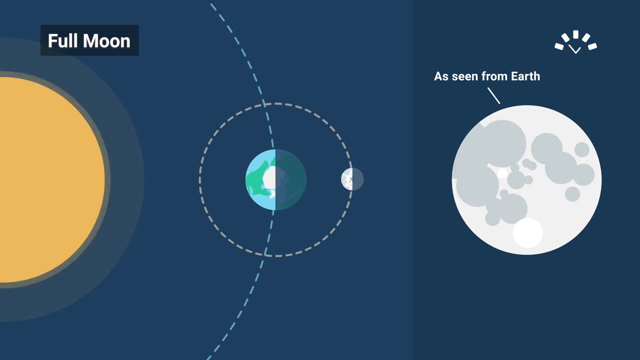 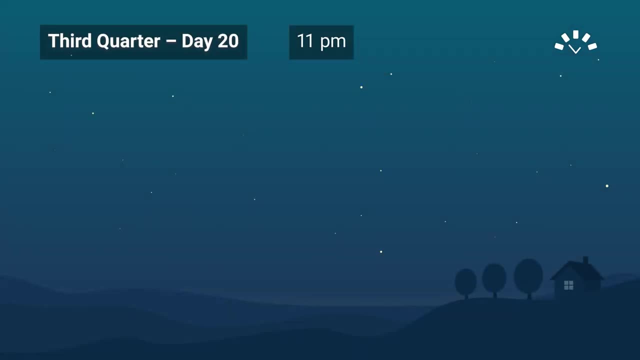 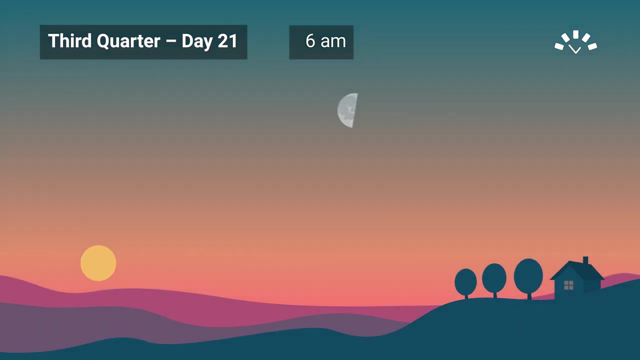 lit up. this is the halfway point of the lunar month and the moon continues to rise later and later. about a week after full moon. the third quarter moon is rising around midnight, as before, half of the moon's face is illuminated, but it's the other way around to the first quarter moon two weeks ago. 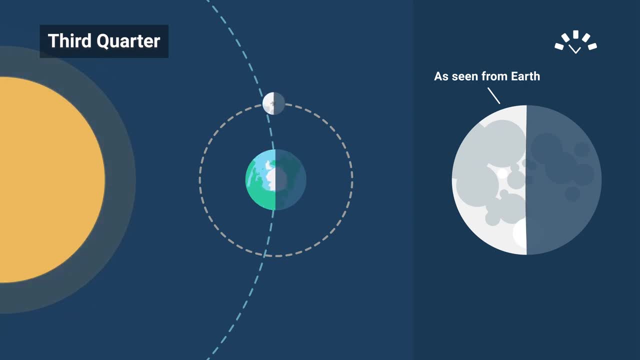 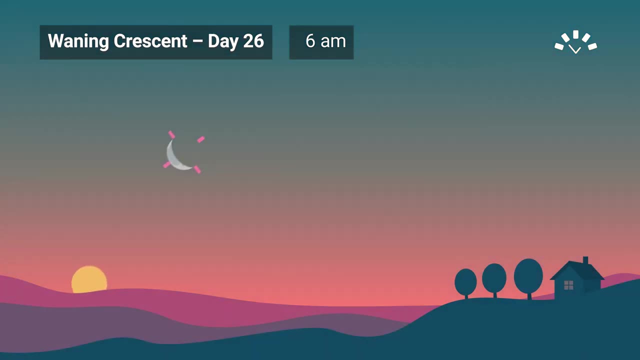 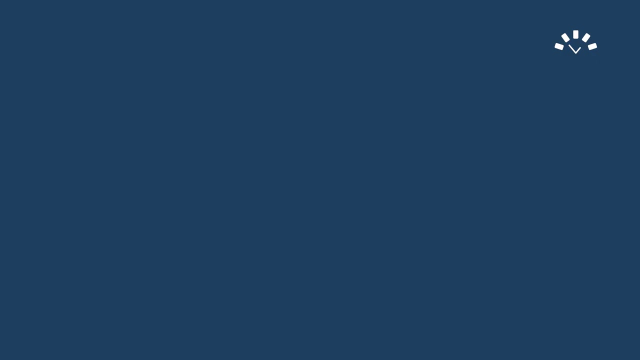 a few days after half moon, it shrinks away again, rising as a thin crescent just before sunrise. and once more the moon is rising again. and the moon continues to rise. it's lost in the glare of the sun. as the moon passes between the earth and the sun, we're back at new moon again. it's been just over. 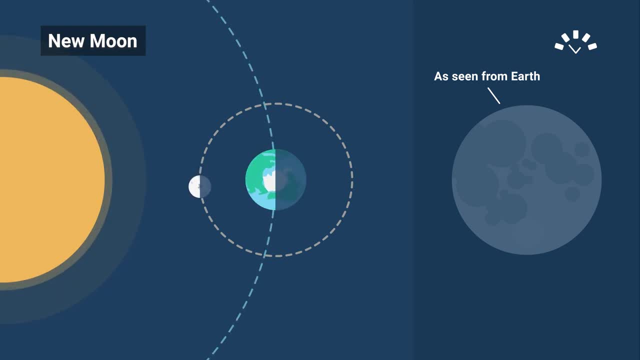 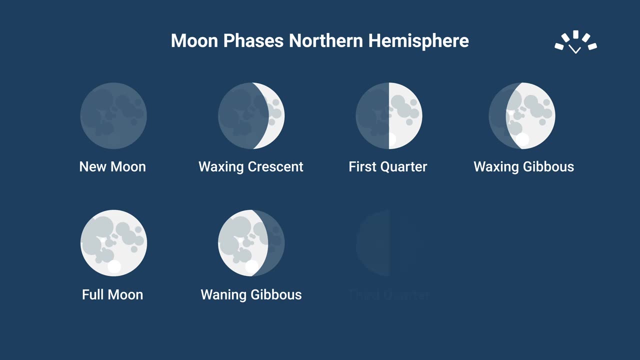 four weeks since the last new moon and the lunar cycle begins again, and now it's over to you. what's your favorite moon phase- a delicate crescent moon, a bright full moon or a quarter moon against the blue sky? tell us in the comments below. tell us in the comments below and we'll see you in the next one.